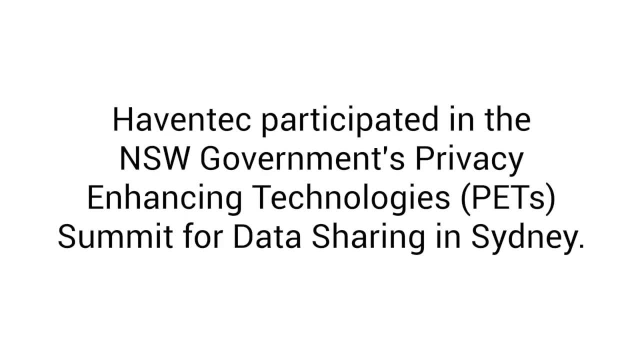 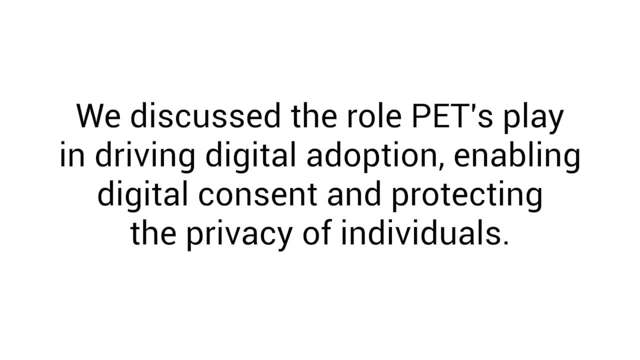 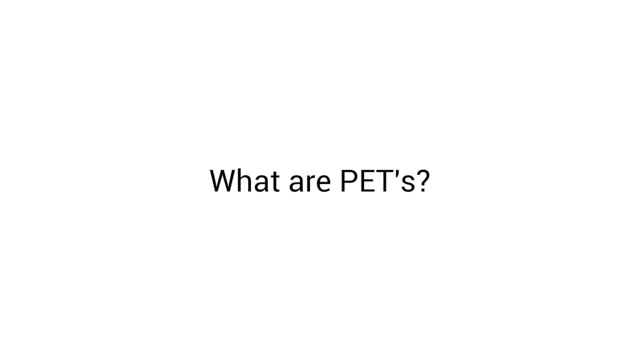 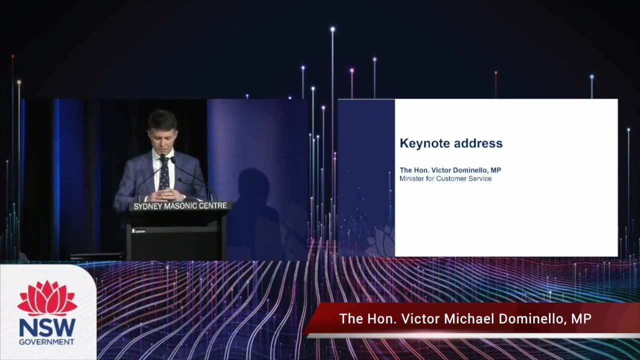 A new industry sector is rising rapidly right around the globe that involves technologies that help companies use data whilst protecting privacy, particularly the use of privacy enhancing technology. These pets are a common weapon and a key weapon in ensuring protection of that data, allowing maximum value to be unlocked from data without compromising privacy and 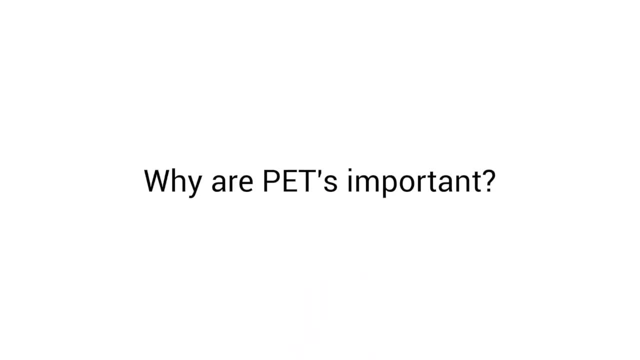 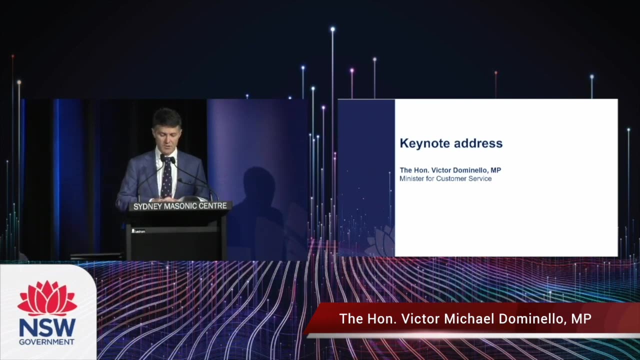 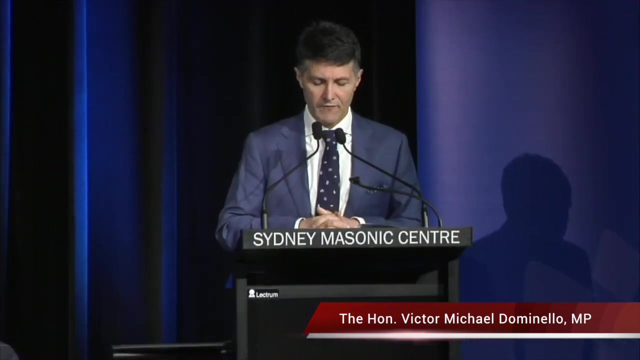 security. By 2023, 65% of the world's population will have its personal information covered under modern privacy regulations. That's up from 10% from today. 87% of customers see benefit in sharing their data right across government. 92% of customers feel comfortable or neutral. 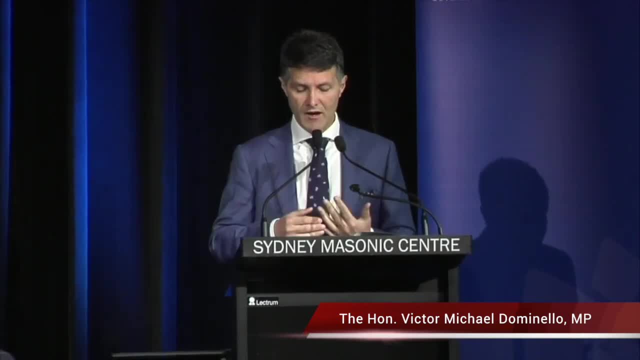 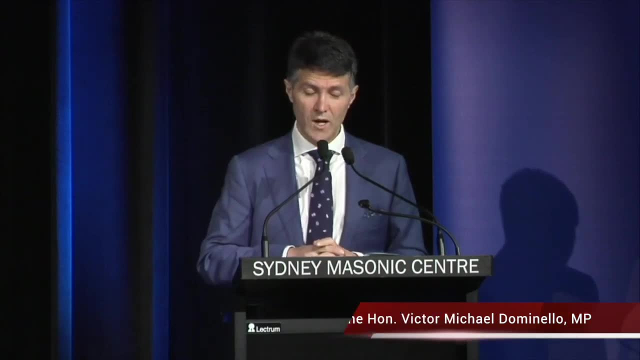 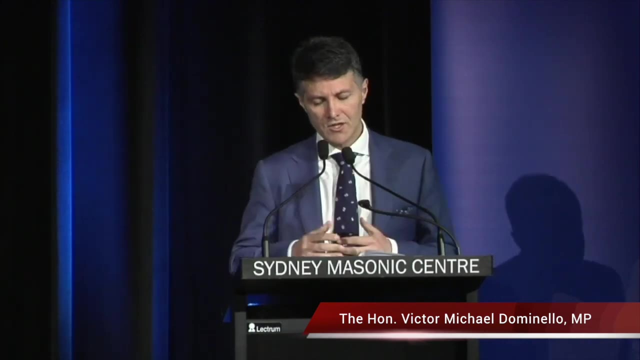 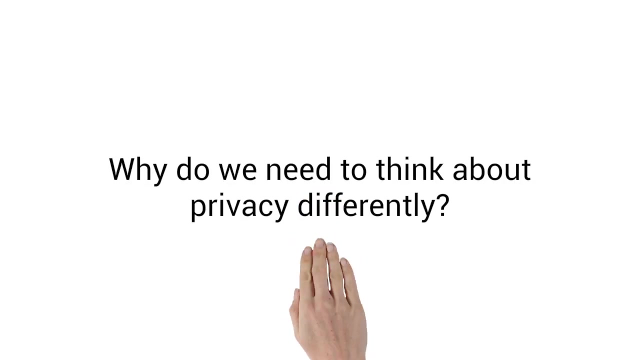 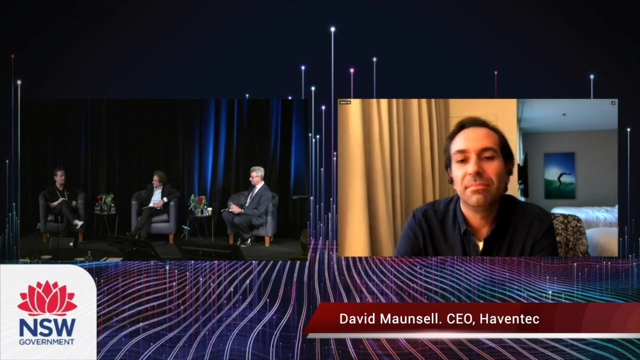 about their personal information being shared within government to make services easier. Traditional ways of protecting shared data often rely on aggregation, averaging or suppressing. Pets go much further, maximising data security and empowering individuals in a number of ways. Current technology and the current technology architectures are providing an adequate protection. 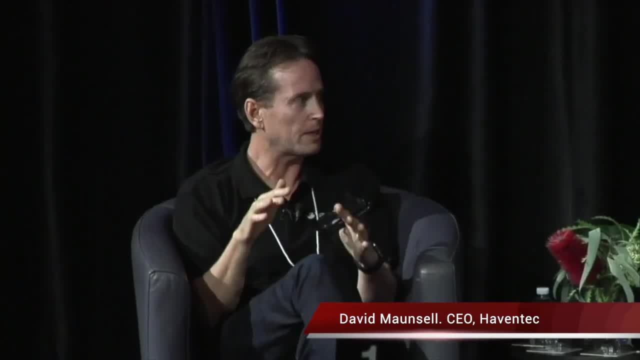 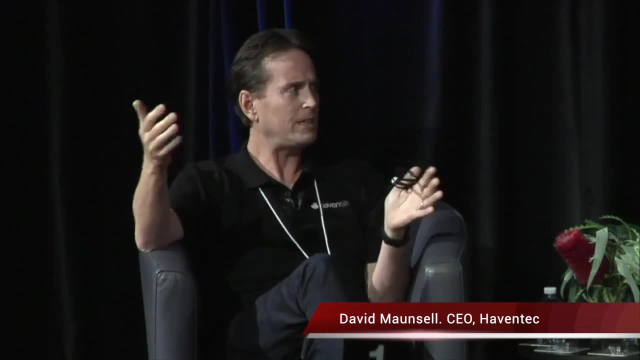 to sensitive information. So if we continue to generate more data, more personal data, off all of the interactions we're having with the digital ecosystem and continue to rely on centralised infrastructure with defence mechanisms sitting around it, I can't see the problem that we're facing. 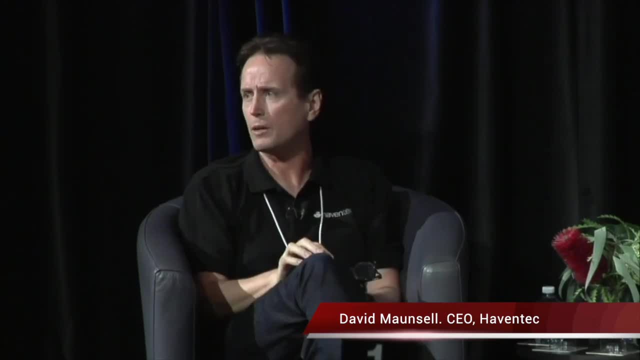 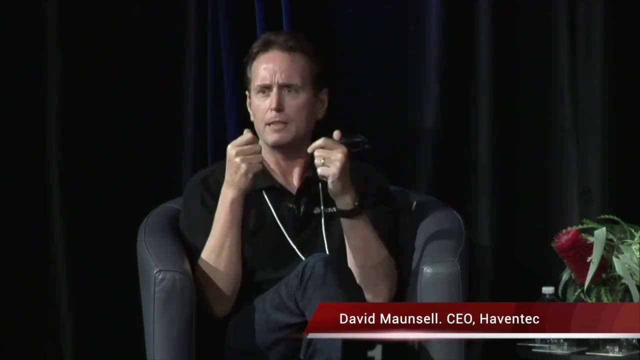 going away In the absence of thinking completely differently about how we go about protecting sensitive information and engaging customers in some form of process where they're consenting in the moment for that private or personal information to be used for an outcome that the brand and that customer is seeking together. 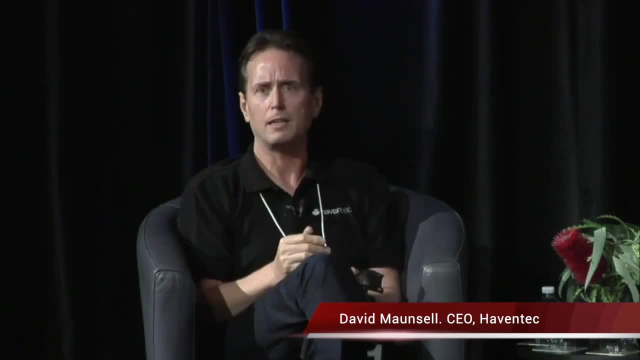 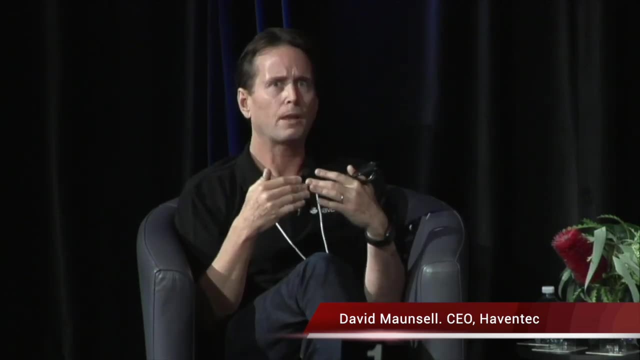 Then we're going to continue to see what we're seeing on a regular basis in the papers: that a whole lot of other data has been lost. So we can't- I don't think we can- approach the future with optimism and hope in the absence.